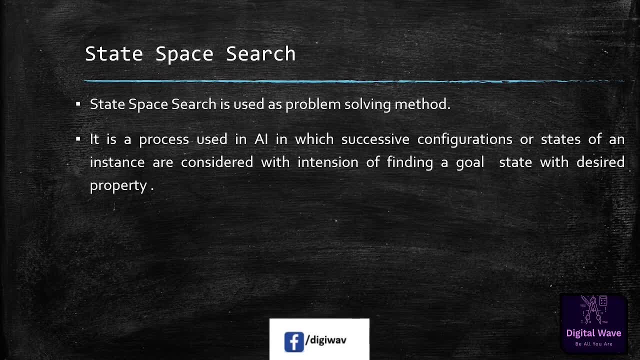 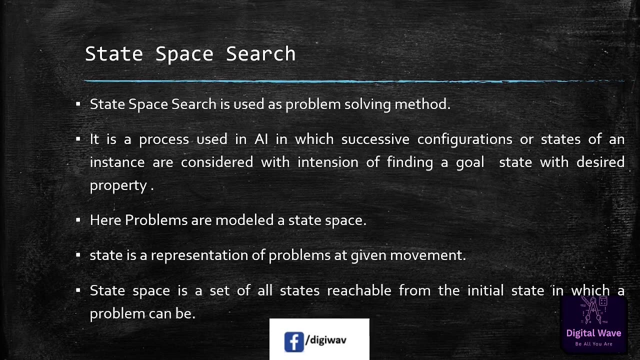 state space search will provide us possible solution of any problem. Here problems are modeled as state space. State is a representation of problems at given moment. State space is a set of all state reachable from the initial state in which a problem can be, So whatever the possible solution will be there. So state space is a group of 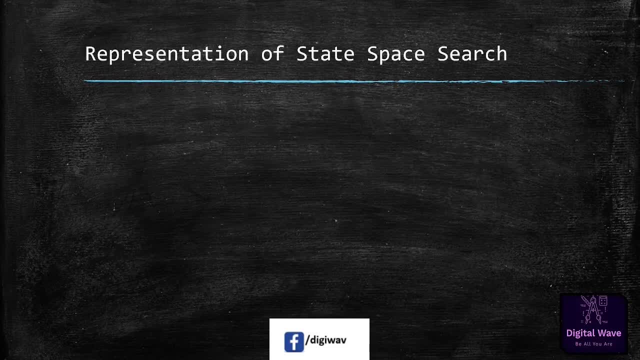 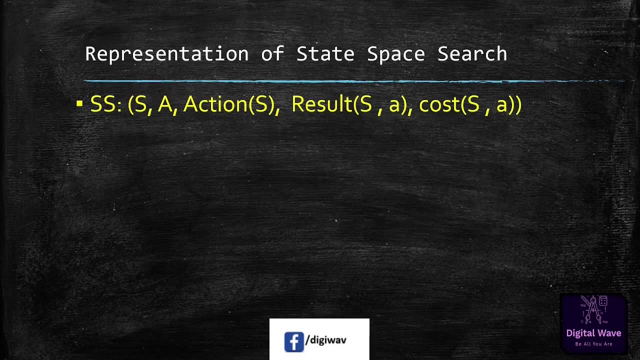 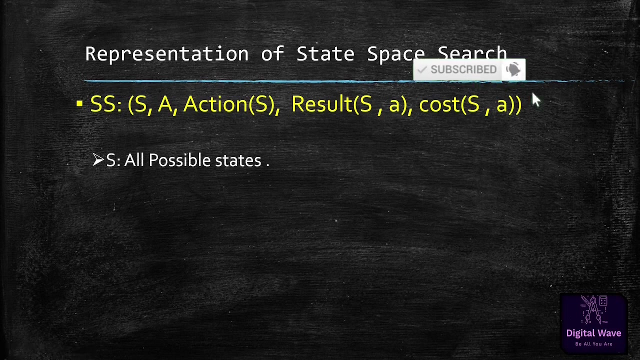 those all possible solutions. After that, representation of state space search. So there is a equation by which we can represent this state space search method. So here this double S is denoting about the state space and this S is telling about the all possible states of any problem. Okay, So if we have any problem and we have to provide the solution of that problem, 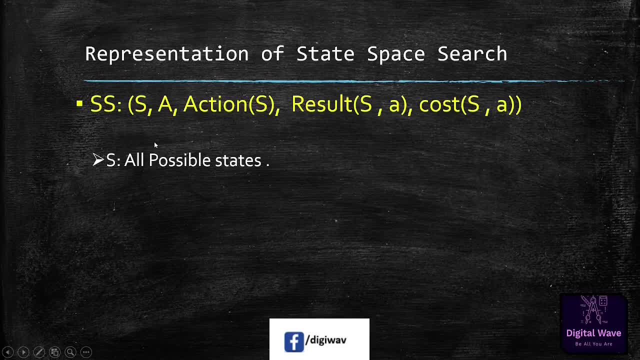 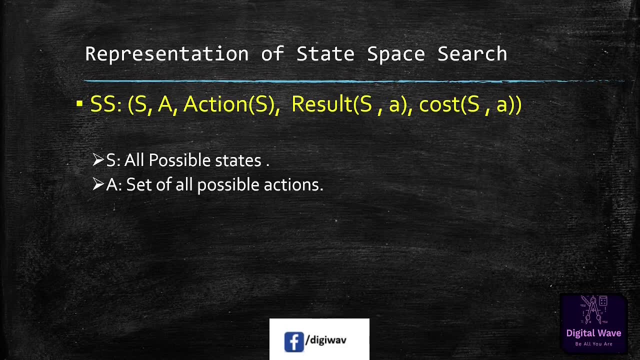 Then this S will represent all possible solution or all possible state to reach the goal state. After that, this A will indicate about the set of all possible action that is required to provide a solution of problem. Okay, So whatever the action we will perform to solve that particular problem, This A will denote that particular actions. 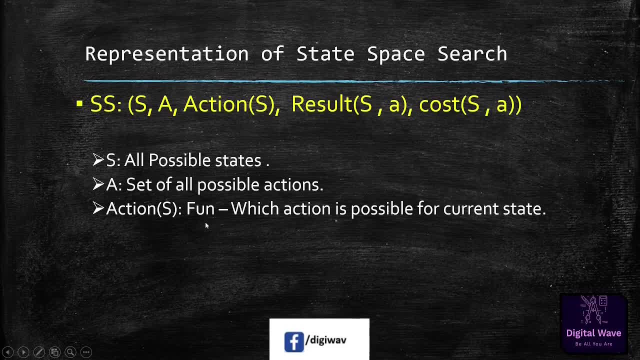 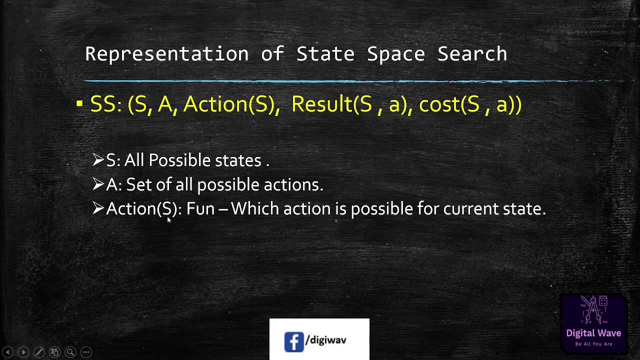 After that, this action. so this action is a function and this will indicate about the all action that is possible for current state. okay, whatever the action you are uh performing on this s or this current state, that this action function will denoting about that particular action. okay, so this action s. 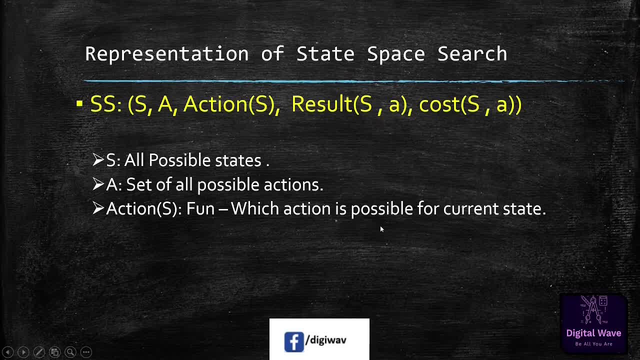 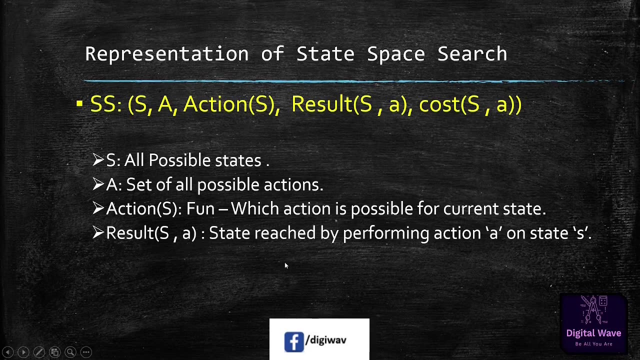 is denoting about the action that is possible for current state. okay, so in current time, whatever the action you are performing on this state, it will denote the same after that result s a. this result s a is denoting about the state reached by performing action a on state s. so, whatever. 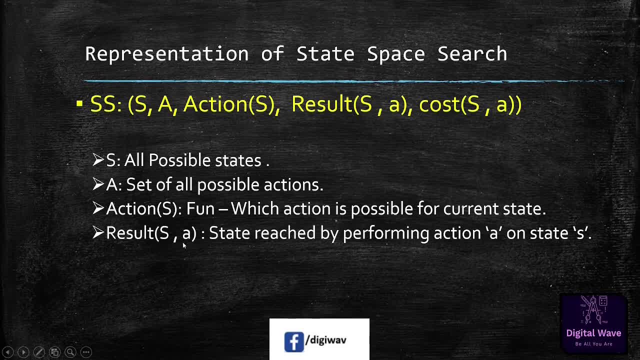 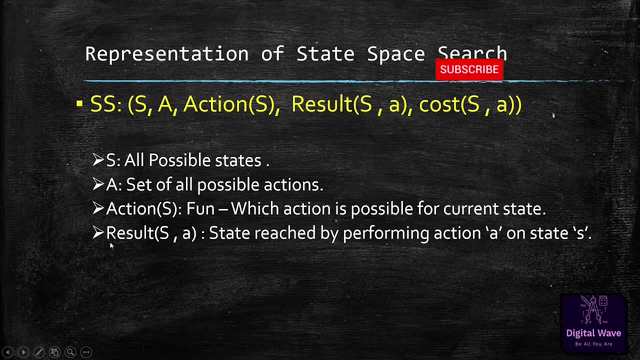 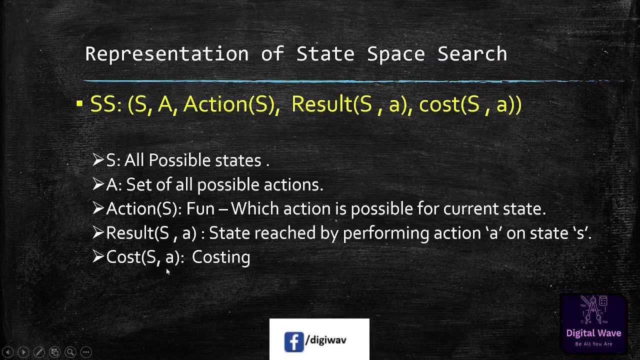 the action you are applying on this state and after applying this action you are getting the result state, then that particular result state will be denoting by this action. okay, so this is also a type of action. after that, this cost s a after applying this action, a on this state. 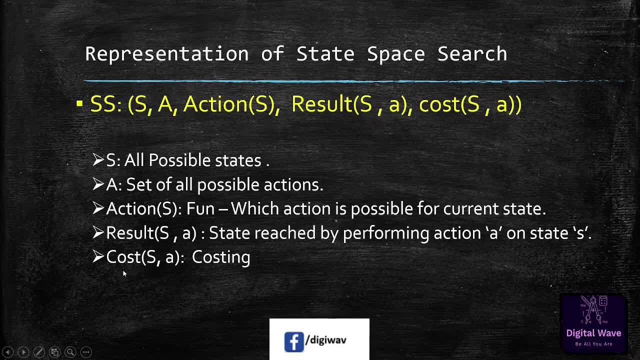 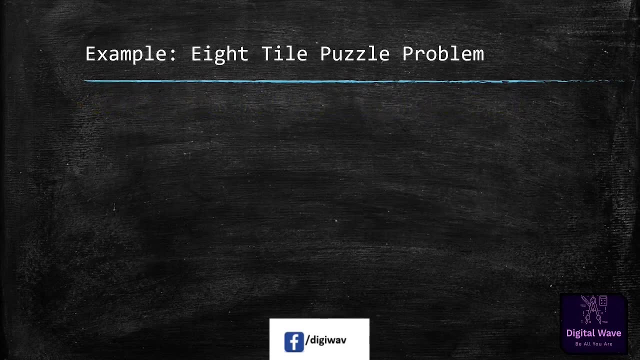 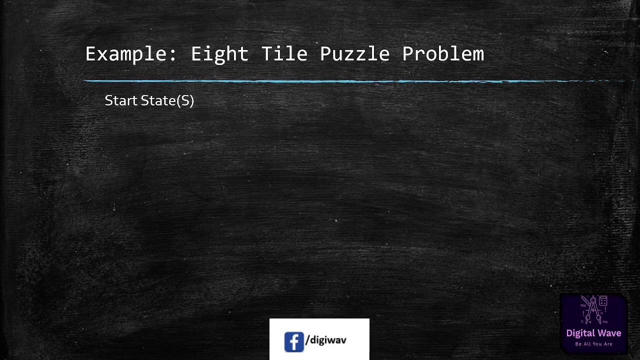 s, whatever the costing you have. that is denoting by this cost s a action. so this is all about the equation that will represent the state space. search in the artificial intelligence, search in the artificial intelligence. now we will understand this state space with the help of this eight tile puzzle problem. so in this eight tile puzzle problem we have 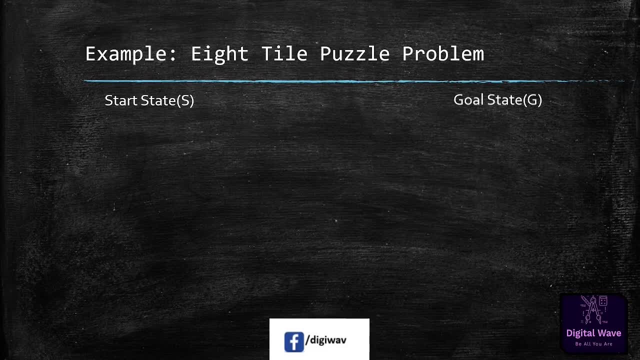 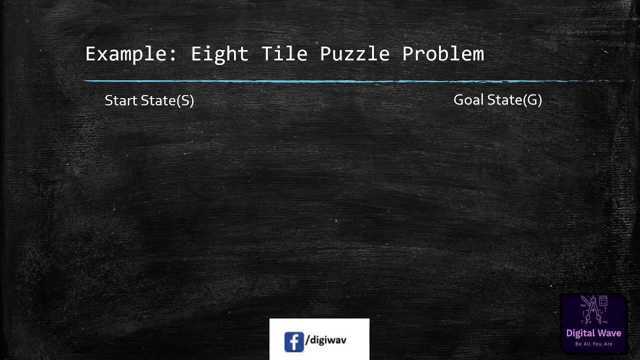 one start state and goal state. so start state will represent about the problem, initial states. okay, what so? whatever the problem you have and whenever you are going to provide the solution, and so in the initial state you will denote that particular state as a start state and the goal state will be: 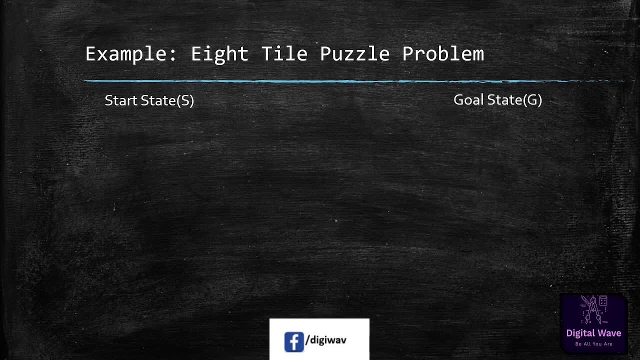 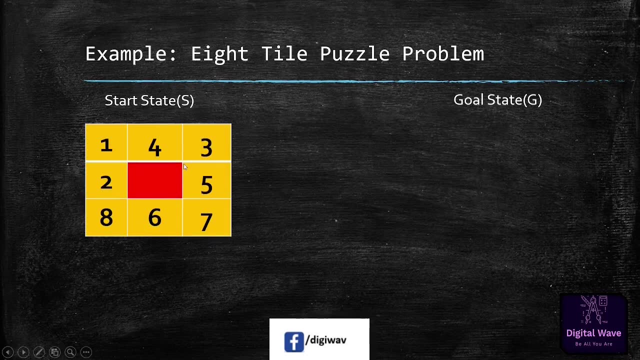 the result of our problem or solution of our problem. so we have this eight tile puzzles. so here i have nine squares and here i have written these random numbers in every block and this is our goal state. so, whatever the numbers i have in this puzzle, so i want to. 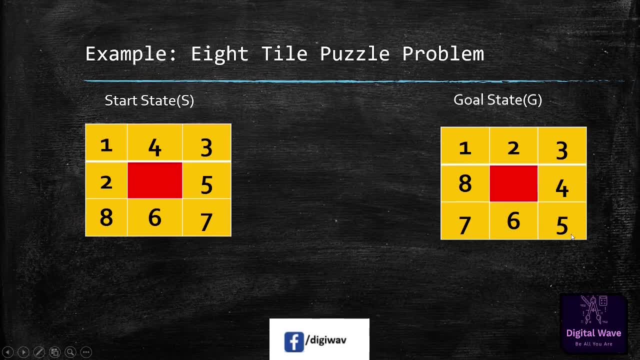 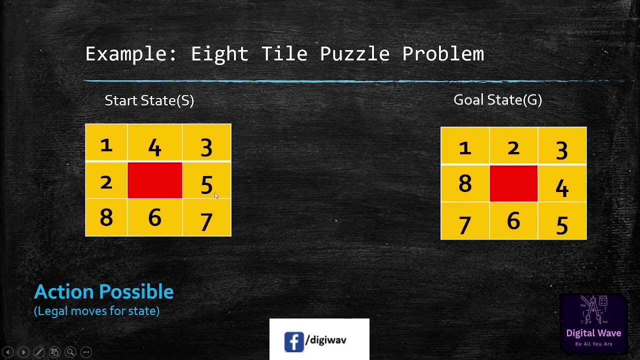 arrange those numbers in this goal state. so what will be the possible action i can perform in on this start state? okay, so we will see what will be the possible action. so legal moves for state. so what will be the legal moves? so here this blank area i have to replace with any number, okay, so 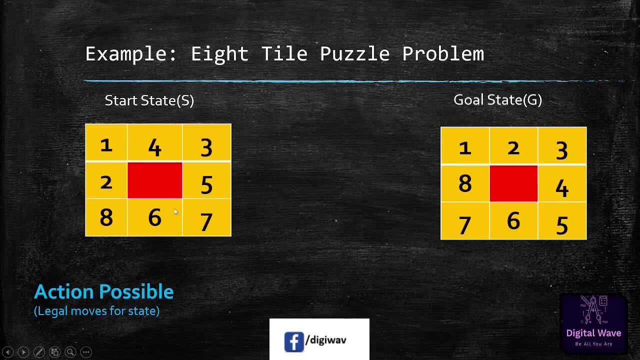 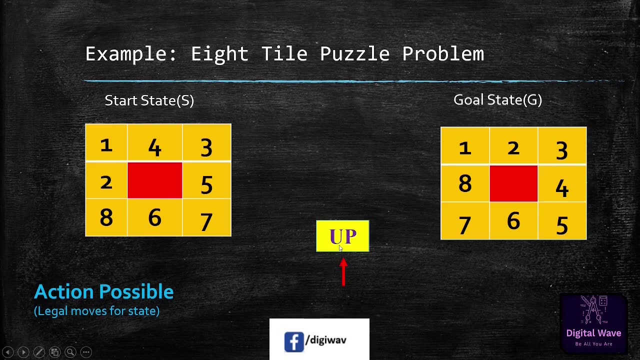 here what will be the possible action. so if i have to replace this blank with any number in this example, here, what will be the possible action? or if i have to replace this blank with any number? okay, so here what will be the possible action i can perform in on this start state so that action will be up if i want to replace this. 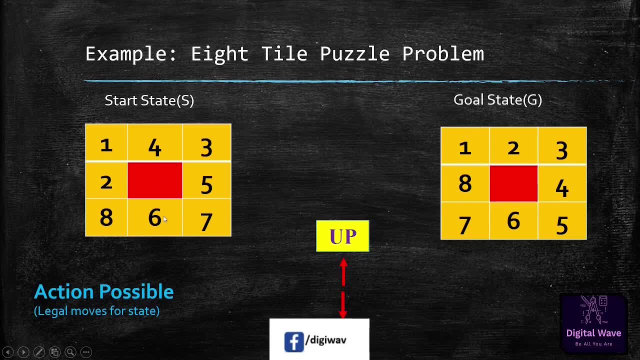 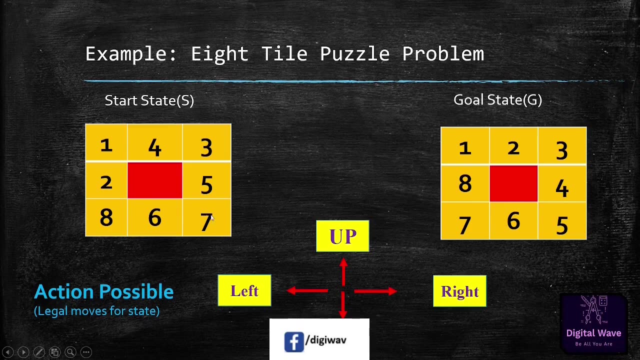 blank area with this four, then we have to perform this up action. if i want to perform this down action, then i have to exchange this with two and if i go to the right, then i have to exchange the value of this blank area with five. okay, so these are the possible actions, or we can say legal moves for the state. so this: 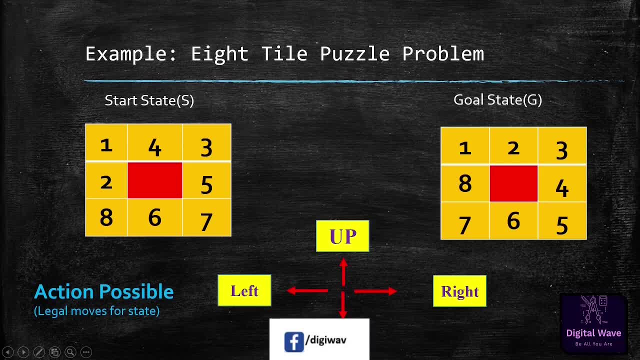 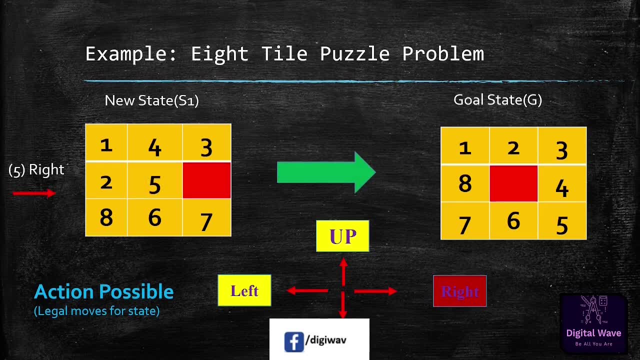 particular state s will have these possible actions. so we will perform every action here and we'll see what will be the result. so, after performing the possible actions, we will get this type of goal state that we have already given in in the form of goal state. okay, 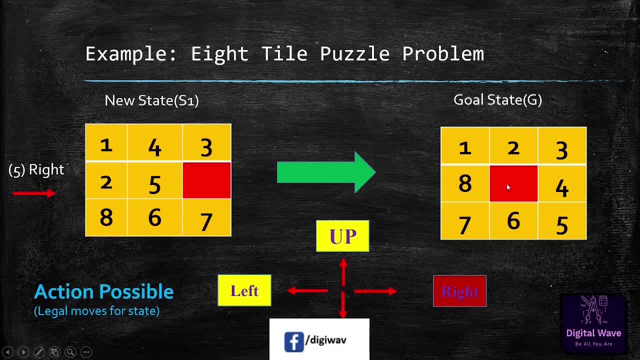 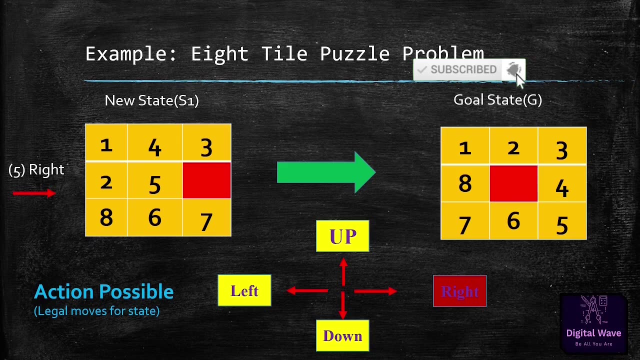 so, after performing all the possible action, we will get this goal state. so this is all about the eight tile puzzle problem. okay, this is the basic understanding of state spirit. so i will take the example of a another eight tile puzzle problem to get full understanding about this problem. so i am taking 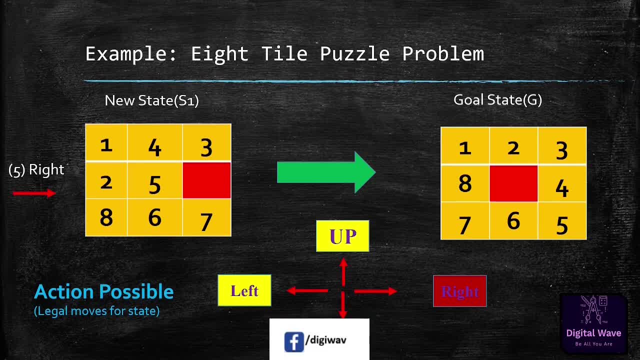 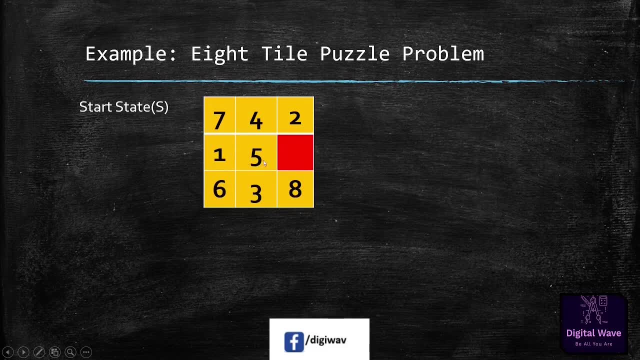 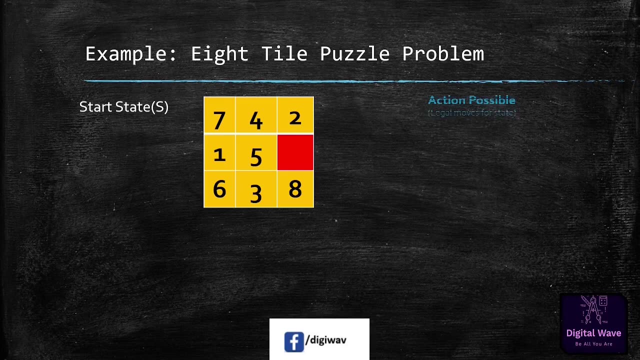 one another example of eight tile puzzle problem to understand this concept. okay, so we have this nine square box and here i have arranged these numbers. okay, so this will be our start state s. after that we will see what will be the legal moves for this start s so up, down and left. so if 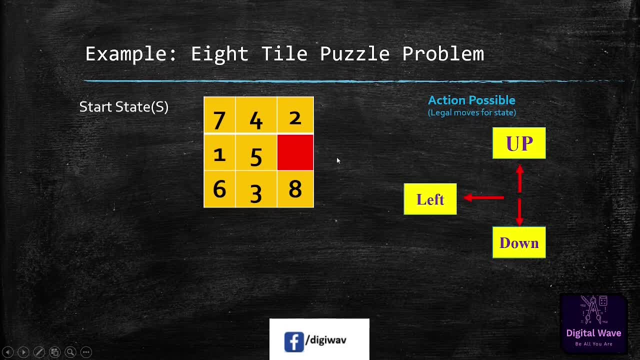 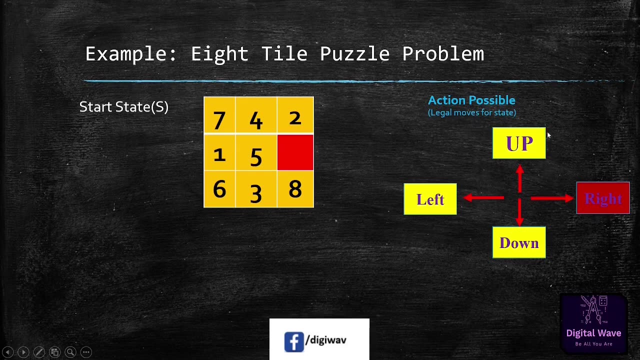 we will see then. we cannot move this state to the right, so right is not a legal move. that is why i have made this color red. okay, so this is not possible move here. so there are three possibilities i can provide to solve this particular problem. okay, so up, left and down. so we will see how these tile 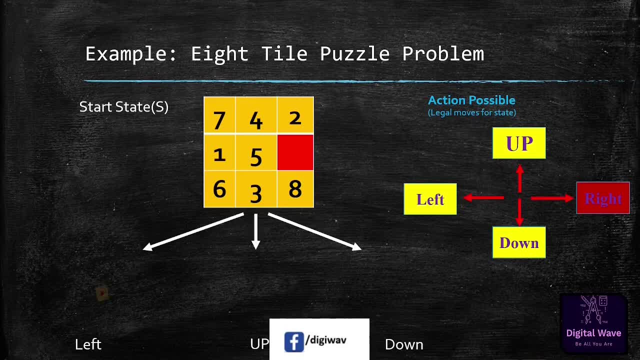 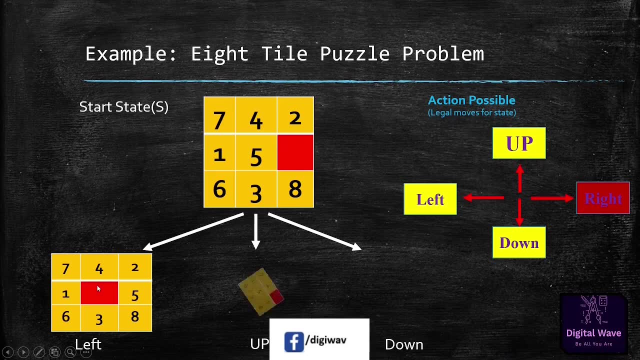 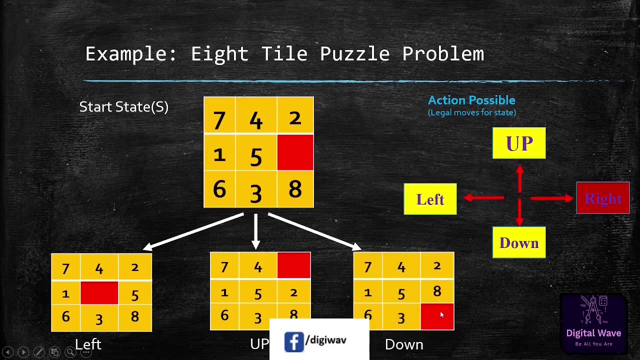 will be after performing these actions. so after performing left, this blank block will be here. after up operation, this blank block will be go up, and after down, this blank block will come here. okay, so now these three solutions, or three solutions, are available. now here we have to solve these three possible solution. we have to 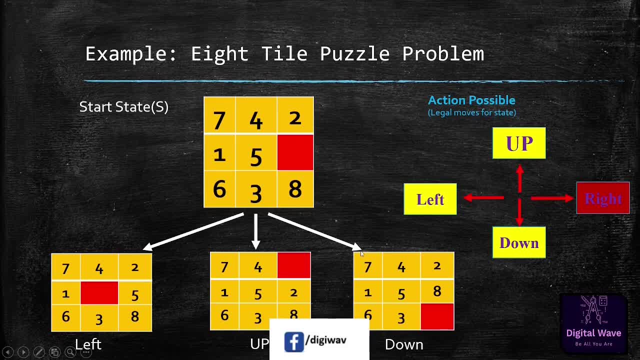 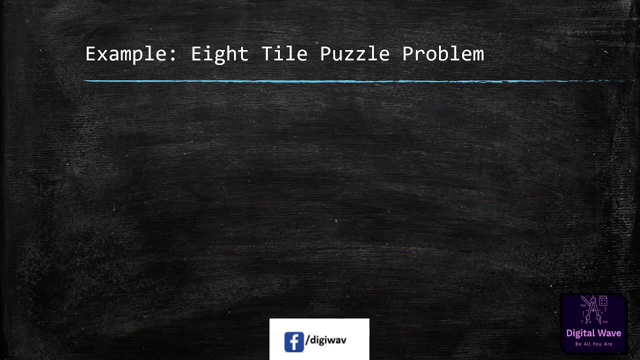 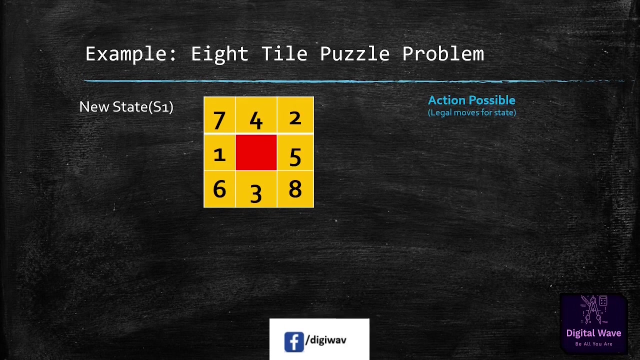 get this problem solution. so there are these three possible solutions. we have to achieve our goal state okay. so here, from these three options, we have to choose one option. okay. so we will keep this left option okay, and we will solve this particular left version. now we will see what will be the possible actions we have. so up will be the 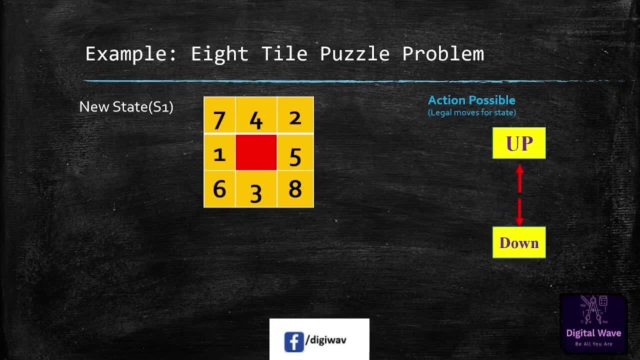 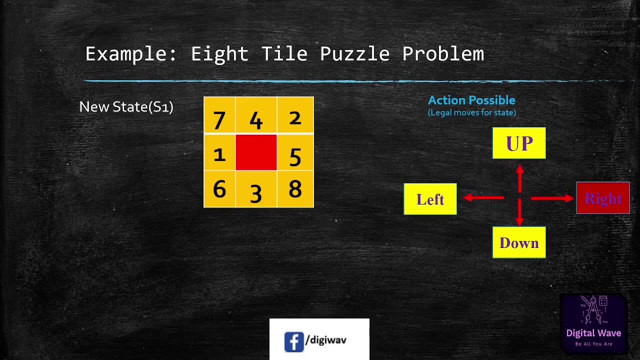 possible solution. down will also be possible. solution left is also a possible solution. here we can see right will be also a legal move. but by performing this right operation we will go in our previous state. okay, so we don't want to go in our previous state because we have to go. 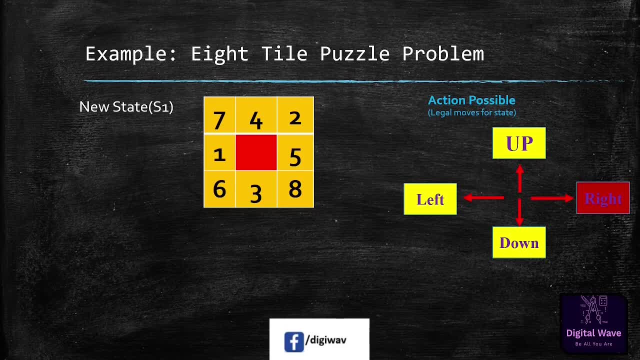 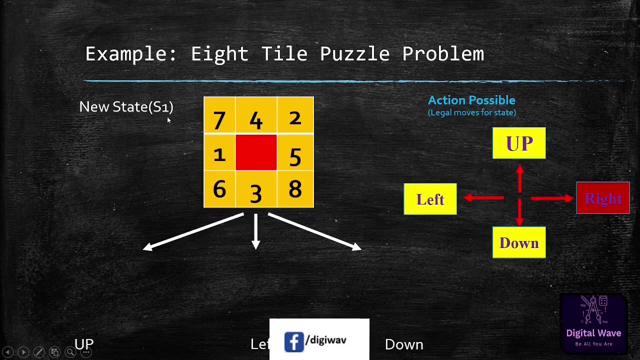 forward to solve this problem. so now we will perform these three actions on this state. now you can see we are denoting this state as a new state, so i have given the name as one. okay, now we will see what will be the possible options available here. so after performing up operation, 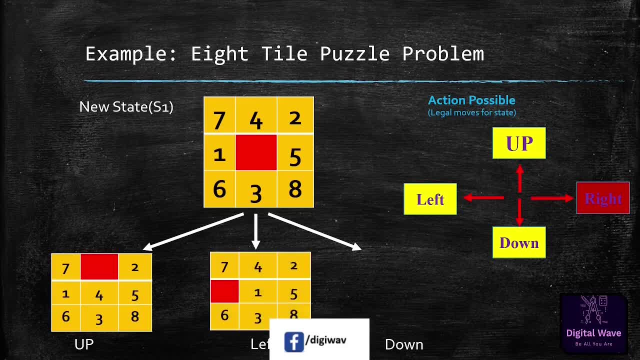 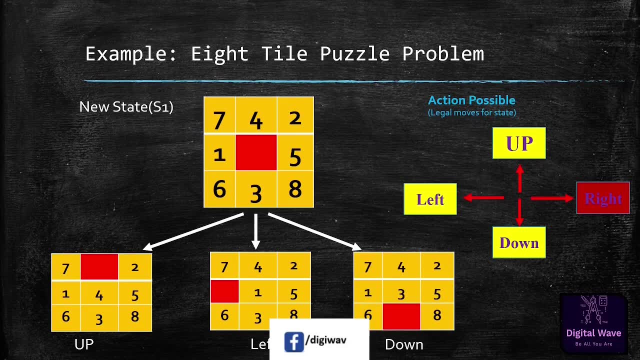 we will get this type, and after performing left, we will get this, and after performing down, we will get this. okay, so now we have to choose one state from these three states, or we can say possible three states. so we will choose one of them and will perform actions. so we will choose. 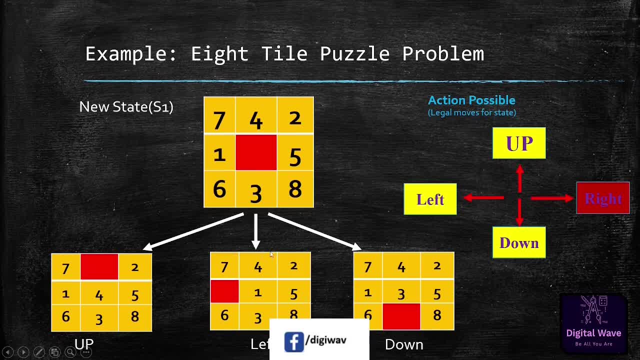 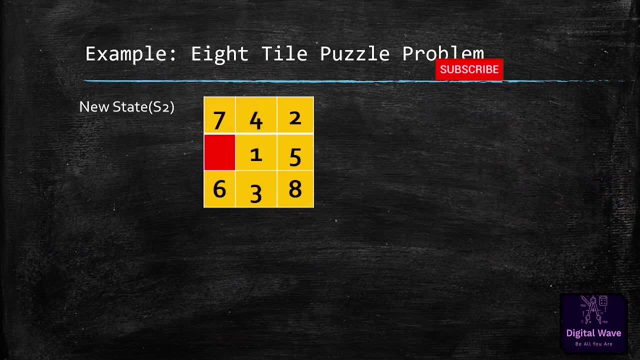 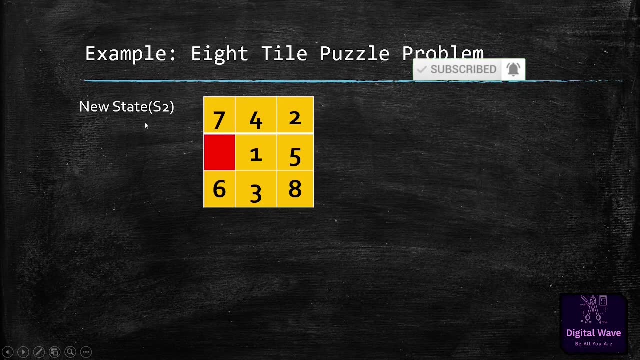 here this state that we have got by performing left operation. okay, so we will take it, and in the next slide we will perform the action on this, a tile puzzle. so now the state is also a new state. so i have denoted this state with the help of s2. now we 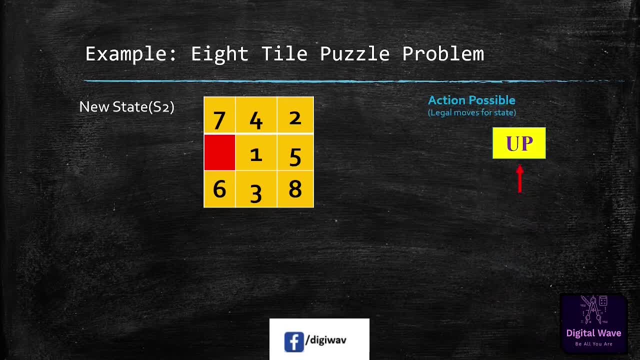 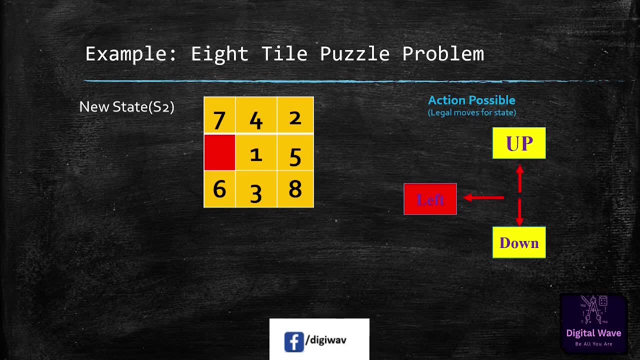 will see what will be the possible action so we can see up will be the possible action, down will also be a possible action. but we will see left move will cannot be possible and if we will select this right, then we will go in the previous state. so we will not consider this right. 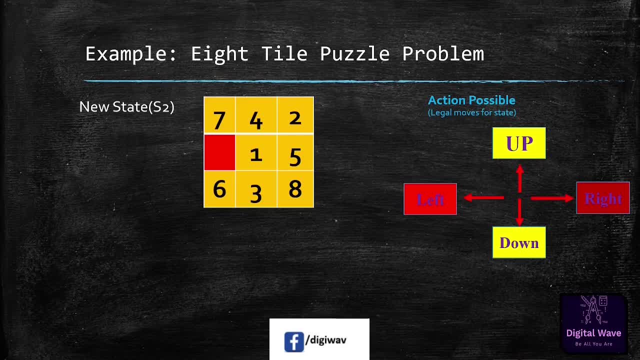 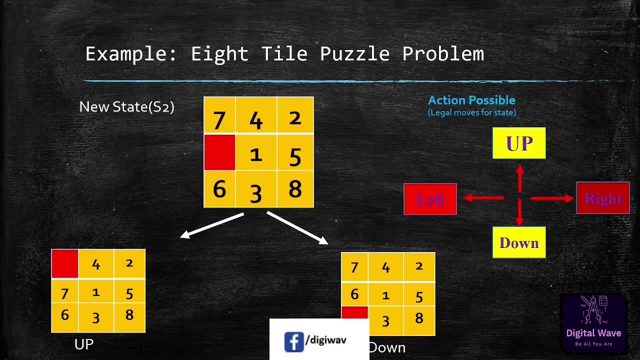 move. okay, now we will go for those two options. so we will see whatever the tiles we will get after performing this up and down operation. after that, we have to choose one state from these two different, different state and we have to continue as we are doing. so, as it is, we have. 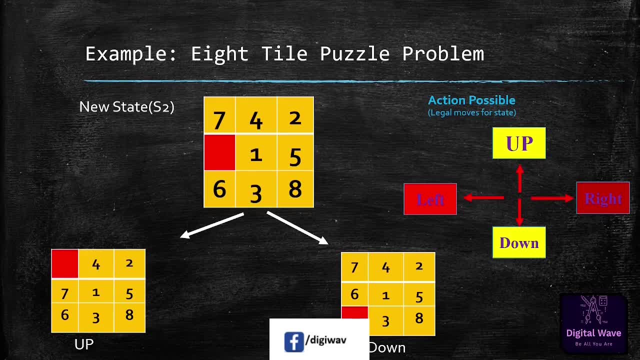 to go further and we will get many other different possible solution. so i hope you have better understanding about this eight tile puzzle problem, as well as this state space search technique. okay, so now what you have to do? you have to give me the possible states to get that particular goal state. 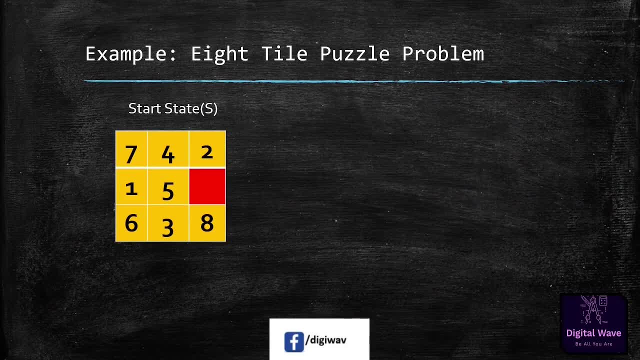 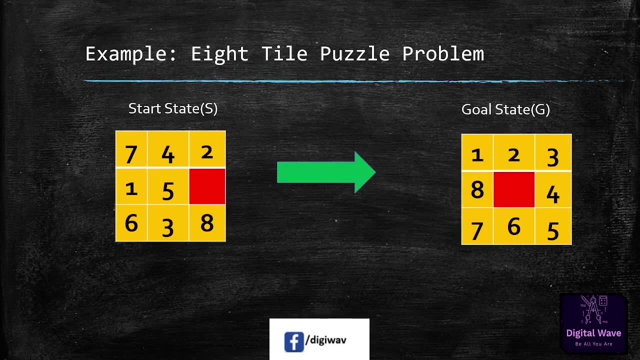 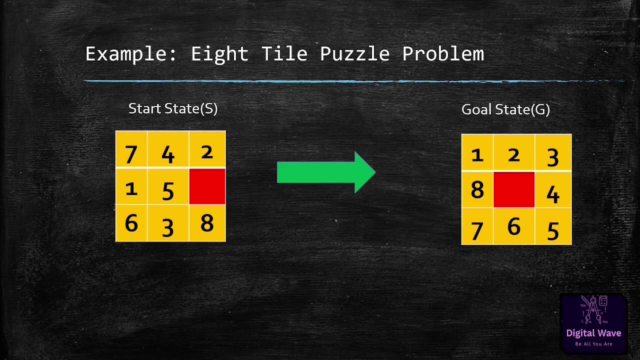 okay, so whatever the initial state we have, and now in how many states or how many possible solutions will be there. so you have to tell me in the comment section then how many numbers of the possible states after performing those actions you will get this goal state. okay, so this is how we can. 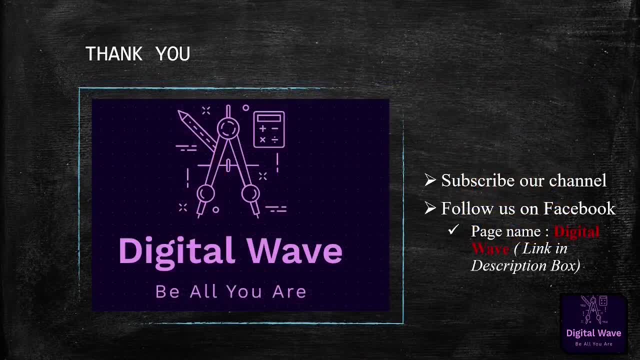 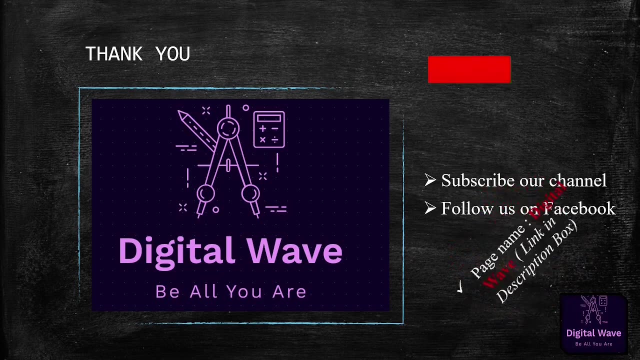 perform these eight tile puzzle problems, okay, so so if you get some information or you get some better understanding about this state space search technique, then please subscribe our channel and we are also available on facebook so you can follow us on facebook. so i have given the link in. 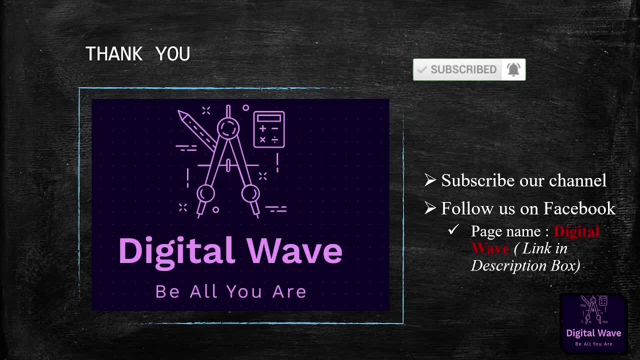 description box by which you can redirect to our facebook page and you can follow our page. okay, so if you like this video, then please share this video and like this video and subscribe our channel. thank you.